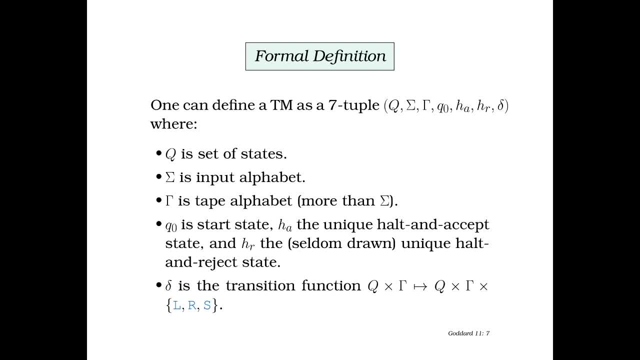 We defined a Turing machine formally as a 7 tupper. So what does that mean? It means it will have different sets. The first is a set of states, which is Q. Now we would be incomplete if we do not have an input alphabet, So sigma represents the input alphabet. 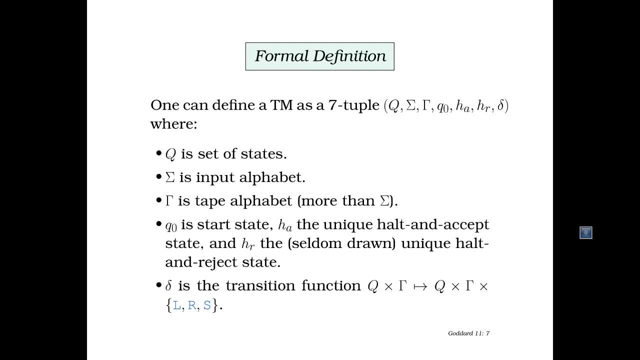 Gamma is the tape alphabet Now. Q0 is the start state, HA is the unique acceptance and halting state, HR is a unique halt and reject state. Now, this is rarely drawn. Delta is the transition function, So it is the cross product of Q and Gamma and results in Q and. 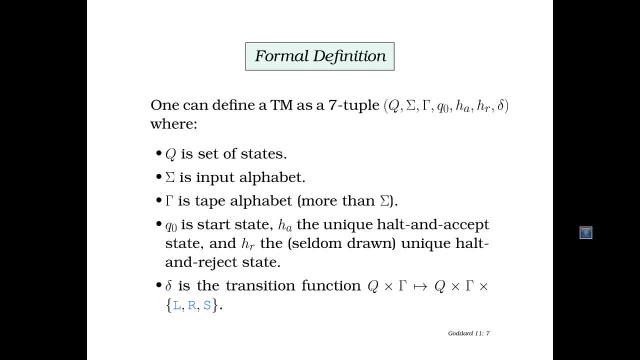 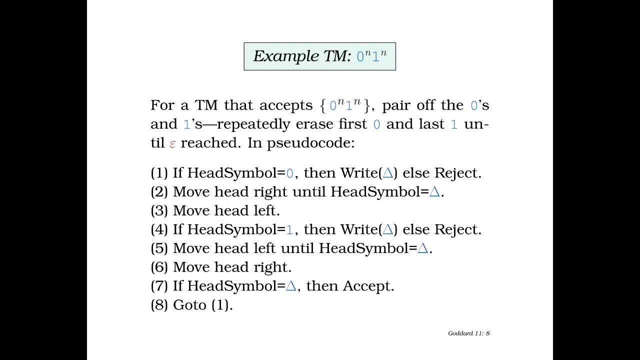 Gamma and either move to the left or right or stay. In this next example we see a Turing machine: 0 and 1n. For this Turing machine, it must accept all strings which have a similar form. So all the 0s and 1s must be paired off. So what we do is we: 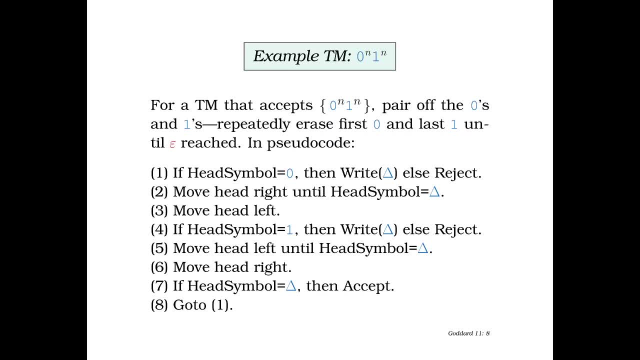 repeatedly erase first the 0 and the last 1 until we get the final result. So what we do is we repeatedly erase first the 0 and the last 1 until we get the final result. So now sing mode 2nd usage: If head symbol x equals 9, if л equals negative, 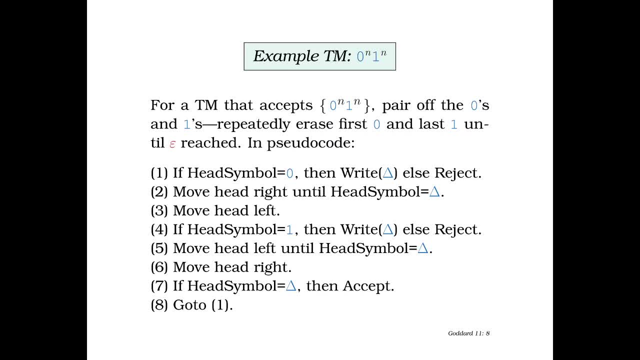 then l is correct right. 3rd usage: We erase this relations tripled. 7th usage: Eggращ can be easily erased if l equals 10 and 1n from the center. so we can see how easy it is to steal the difference between. 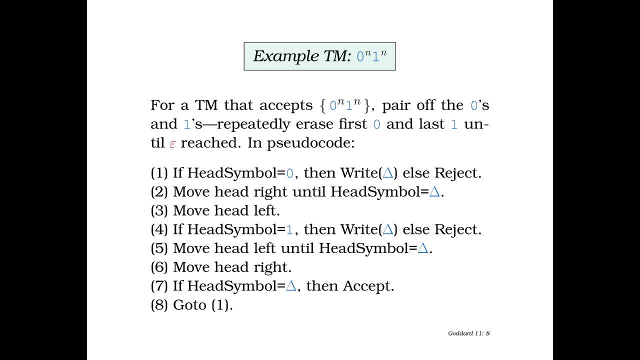 the elements: 8th method On the ordering line, the producción sequence 1. register 2. subjects 9th: 2nd warriors TD 8th- 2nd warriors TD 8th 2nd形 9th. 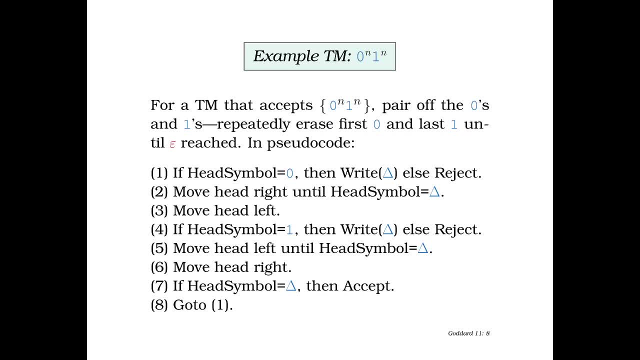 10th, 9th, Sat, Сегодня, 10th Actual 9thmit 10thw 9th. 2nd, move head to the left until head symbol equal Delta, move head to the right and finally, if head symbol equal Delta, then accept and you go back to one. so if you, 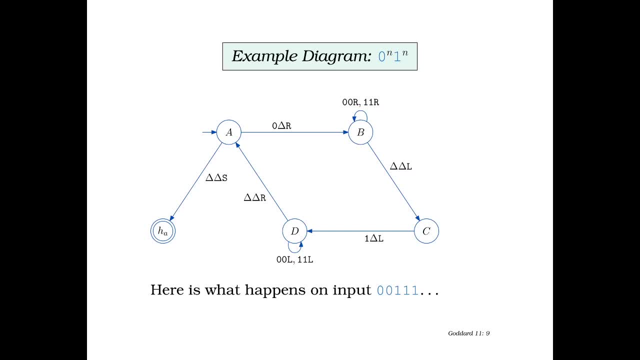 look at this diagram. you see, we start with the state a. in case of a zero, we replace it with Delta and move the head to the right. we also move from the a state to the B state. now, likewise, if we are in the B state, we can encounter a. 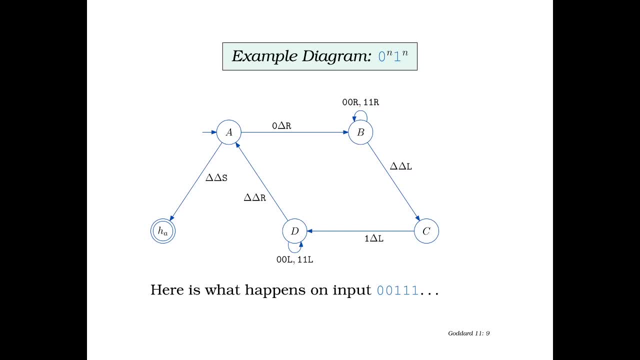 zero or a one or a Delta. if it's a zero or one, the head will move right, but if you get Delta, then you move to the left, and so on. so we can look at an execution of this during hint on the string 0, 0, 1, 1, 1. so first, what happens is: 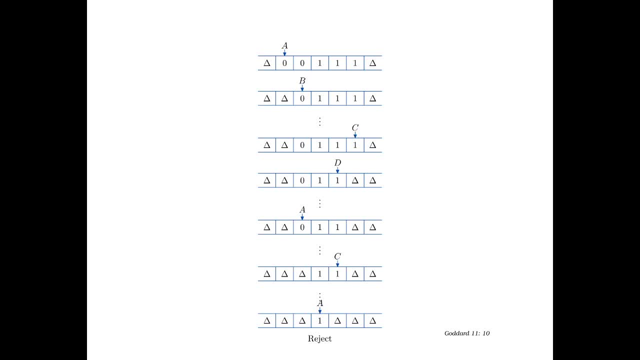 we start with the state a and the head is pointing on 0. now we move to the state B. 0 has been replaced by Delta, and this keeps going till we get to the point in this next position, where it's the state is C, we're pointing to 1, so we 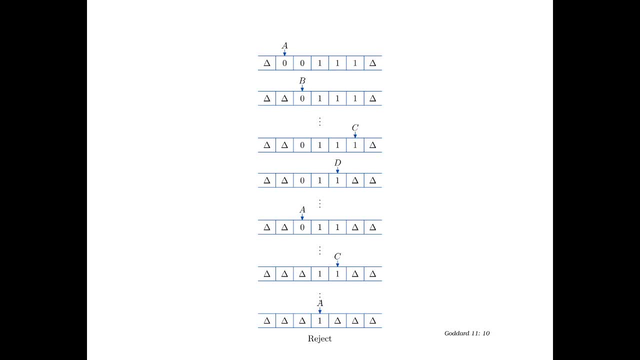 write down our Delta and then so on. finally, we realize that we've written a lot of deltas, but we're still left with one, which means it is a reject. now there are turning machines which simply do not hold. here's an example of a tuning machine. you see there's no accept state here. so what happens is it keeps moving. 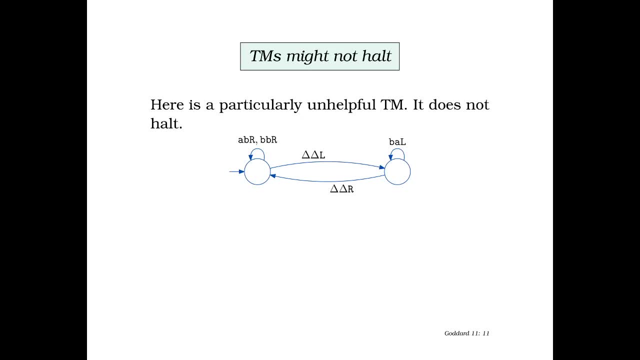 back and forth between the two states, on and on. so it's obviously from this diagram that there is no accept state. so it's will never halt, either for accept or for reject. another example: Turing machine is for balance brackets. what are balanced brackets? often time in programs we need to find the balance brackets. so you have. 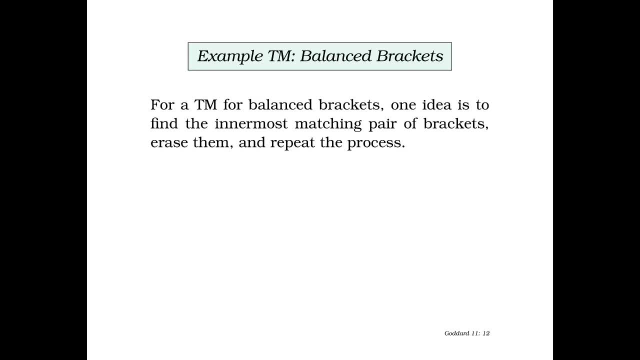 to match that innermost matching pair of brackets, erase them and then keep coin. so for this process we have to use a special symbol to indicate an erase bracket. in this case the example given here is of X. so whenever we want to erase a bracket we write down X. so if you see here it looks a little bit weird. 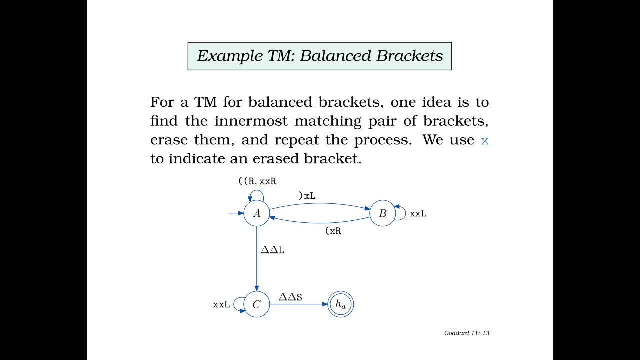 but it's still a Turing machine and it's written in the same notation. so if you encounter the left bracket, you write it down again and move to the right. if you encounter is X, then you let it be there and then move to the right and the state. 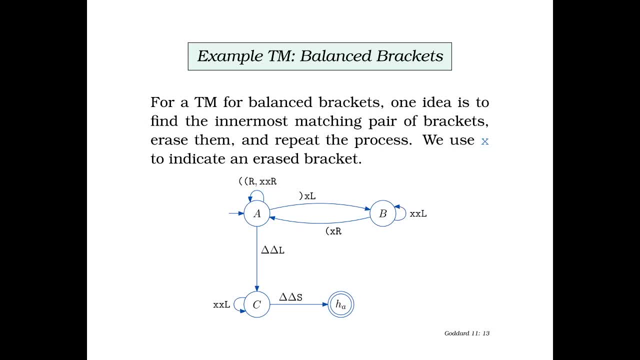 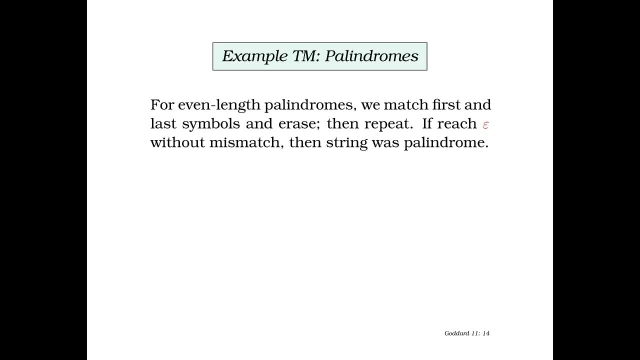 in both cases remains the same and likewise this keeps going. another example is that of palindromes. in palindromes, if it's even length, so we first match the two symbols on the side, so the first and the last symbol, and erase them, then keep repeating if we 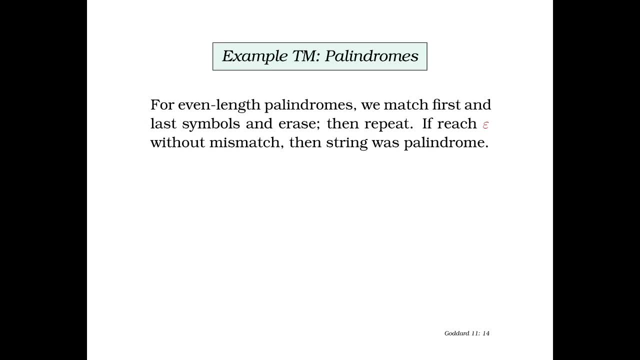 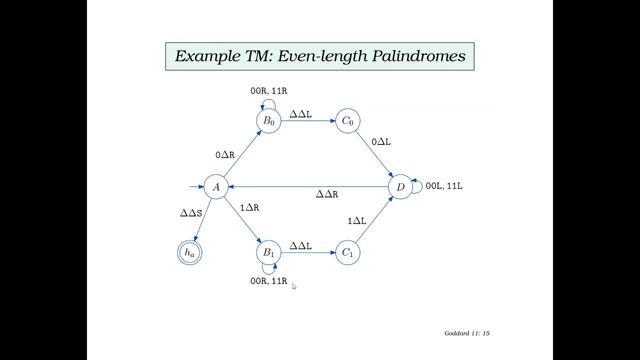 reach epsilon without mismatch. it means the string is a palindrome, so in case, common terms can be solved. so let's look at an example. Turing machine here would see the different states: ab0,, c0,, b1,, c10 and d. The way this machine works. 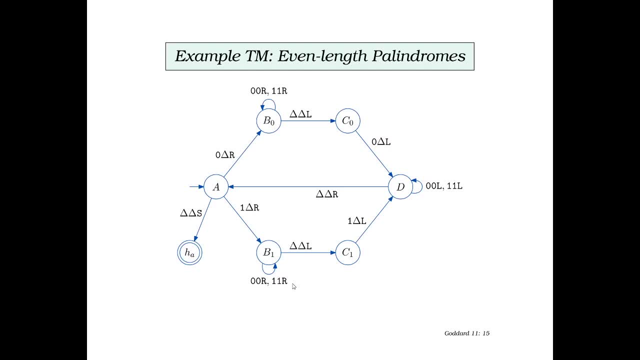 you start out with the state a. if you encounter a 0, then you write down Delta and move to the right. if you encounter a 1, you write down Delta and move to the right. and if you encounter Delta, then you also write Delta and stay, and then. 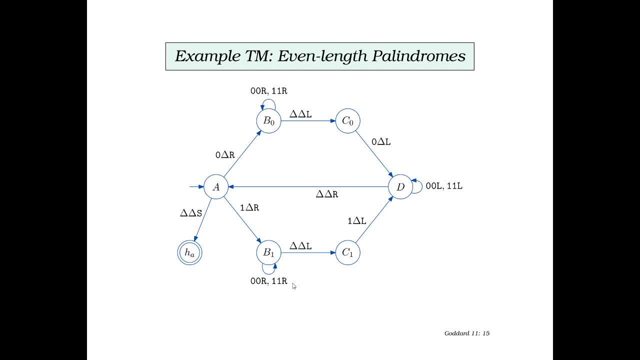 you move to the accept state. as you can see here, in this machine also, not only does the head move to the right, left or stay, the machine also moves from the states. now we do not represent the state of the machine as the state of the machine. we represent a Turing machine, always using diagrams, an easy way to represent. 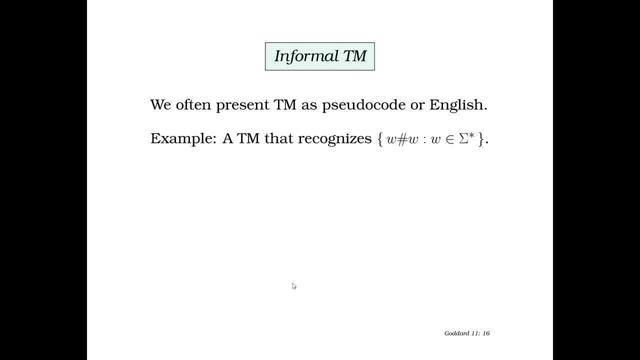 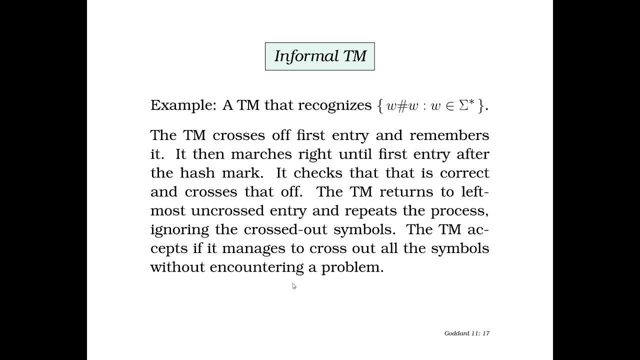 a Turing machine is to write down its pseudocode, which is plain English. so let's look at an example Turing machine, a machine that recognizes a common problem, a language, W, hash, W. so there are two words and they are the same and they are separated by a symbol: hash. so if we look 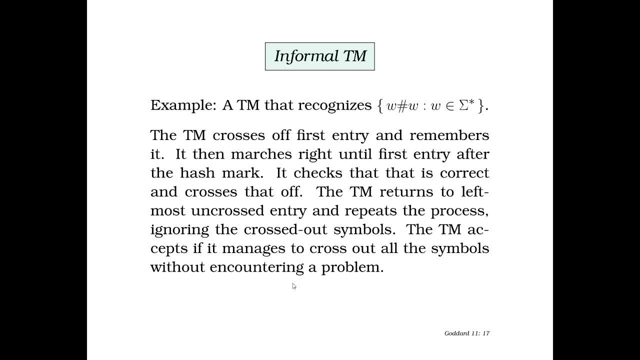 here. how this works is it essentially moves so that it finds the first entry, crosses it off and remembers. then it starts moving to the right until the first entry is fully road and then it reads and responds with the someone. but once the first entry is nothing and it starts Young, and then it recipients the. 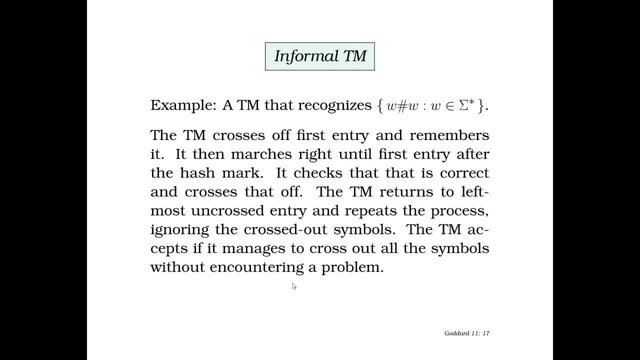 found again after the selected symbol, which is the hash mark. If it is correct, it crosses that off, returns back to the leftmost uncrossed entry and the process repeats itself. It ignores the crossed out symbol. So this Turing machine it will accept if it is able to cross out all the symbols without 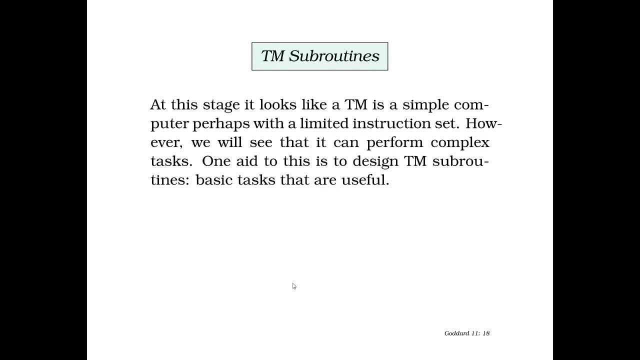 encountering any problem. Now, if you look closely at a Turing machine, it does look like a small computer, maybe with a limited instruction set. However, we can see that it can certainly perform complex tasks. Now, if one aid to that is to design a Turing machine, 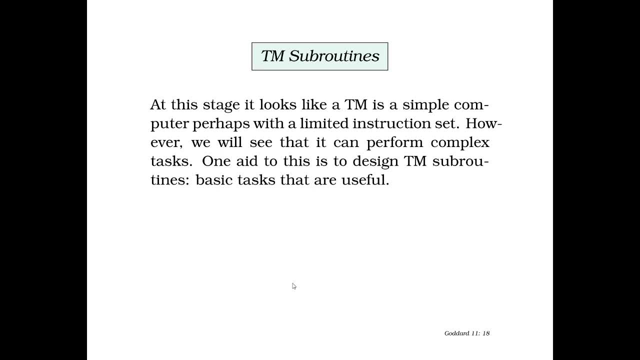 So what that means is that we have some basic tasks that are very useful and we design them The Turing machine for these tasks that would really help us. Let's take an example: subroutine Now. this subroutine shifts the inputs time entirely One cell to the right. 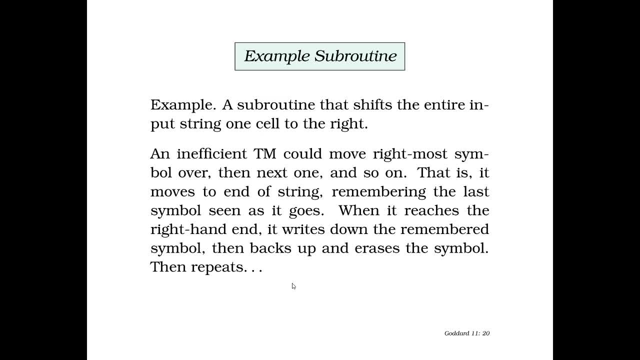 So we can make an inefficient one or we can make an efficient one. If it were an inefficient one, it would move the rightmost symbol over, then the next one, and so on. That is every time it has to move to the end of the string. 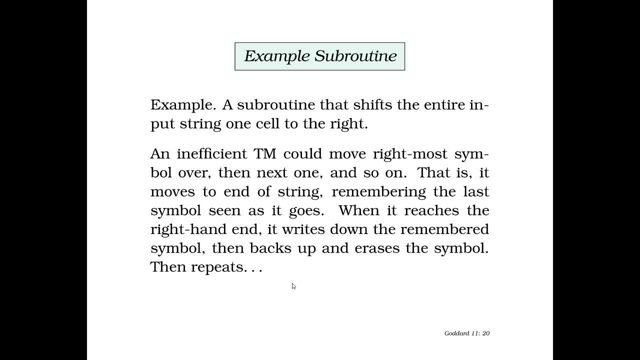 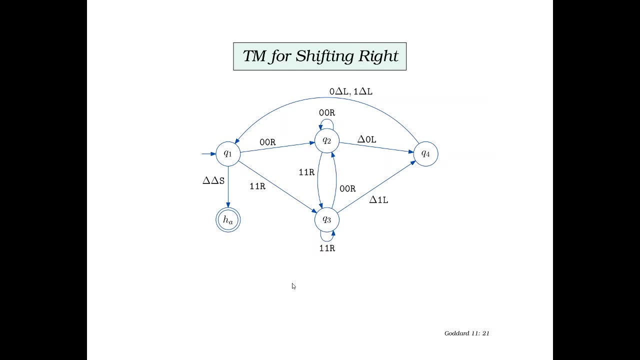 Remembering the last string, the last symbol, as it goes, and when it reaches the right hand, it goes right down to the remembered string, backs up, erases the symbol and keeps going. So this is an example implementation. We have certain states. we have the accept state, which is represented by HA. 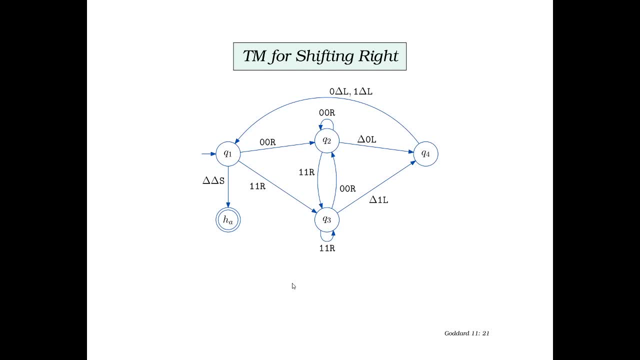 So when we start out, we have three options. Our state is Q1. So we can either move to Q2, Q3 or to the accept halting state, depending upon what we are seeing with the head. If we see a zero, then we let it remain there on the day and the head moves right and we